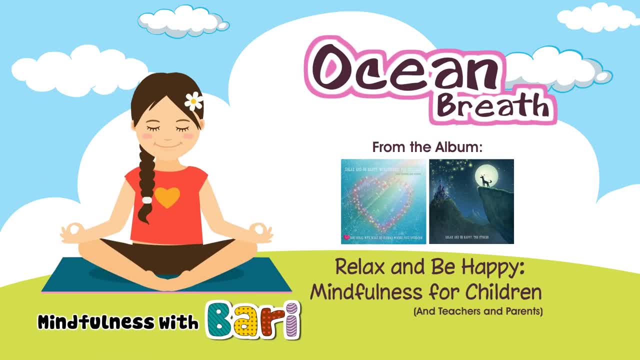 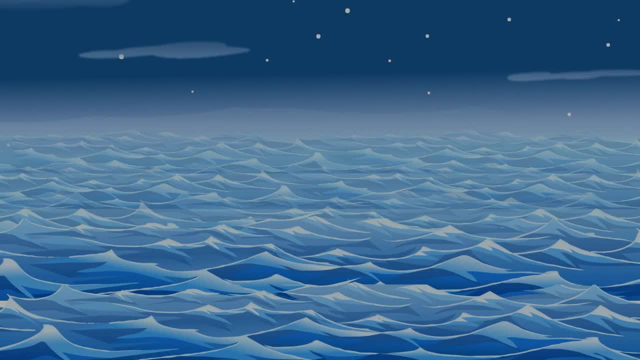 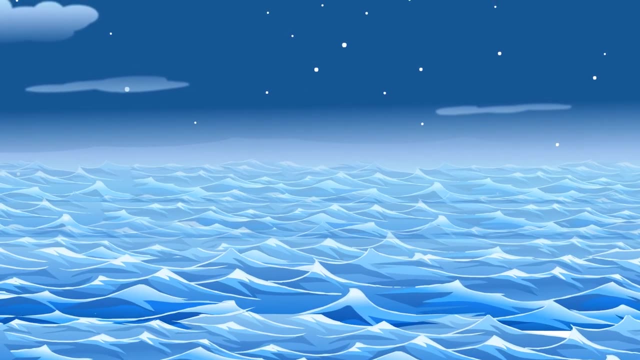 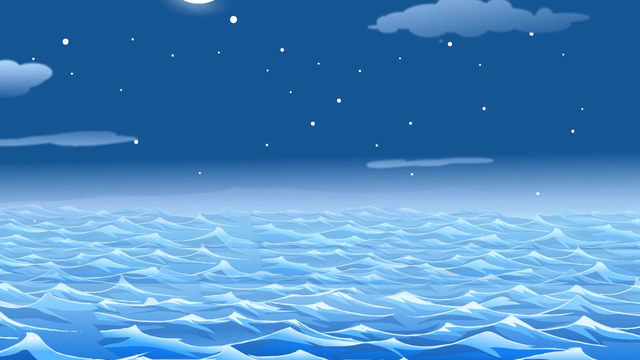 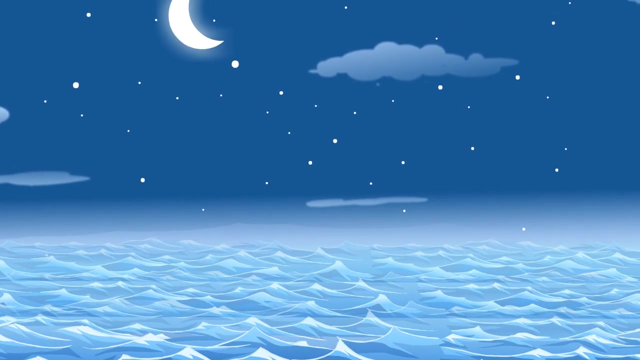 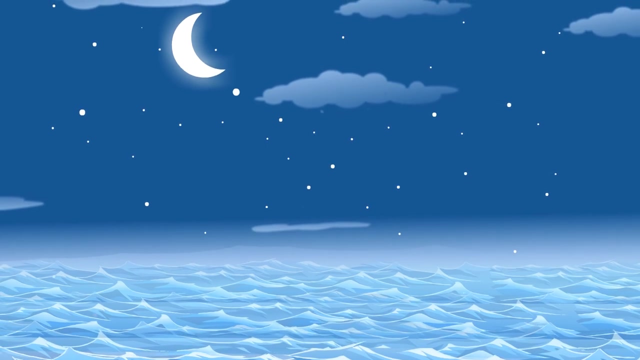 Close your eyes and imagine your belly is full of water like the ocean. Inhale, let the waves rise in your belly. Exhale. let them fall. Inhale, let the waves gently rise And exhale. let the waves fall. 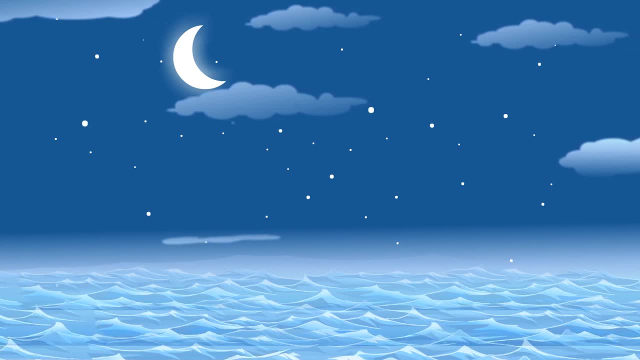 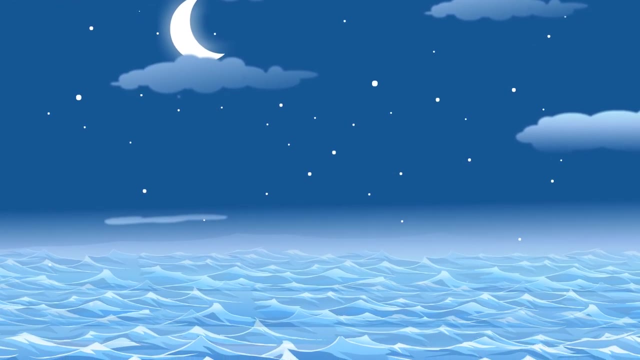 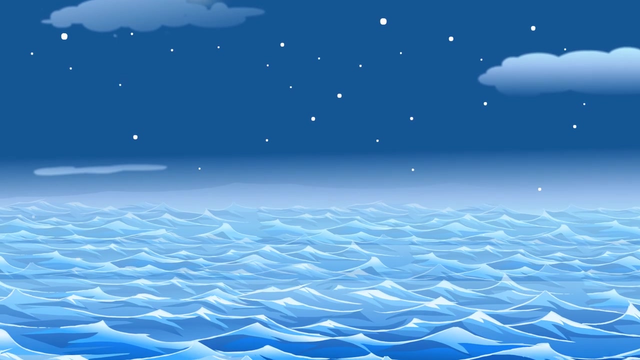 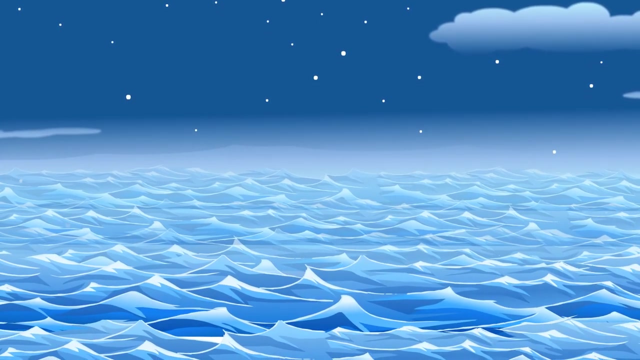 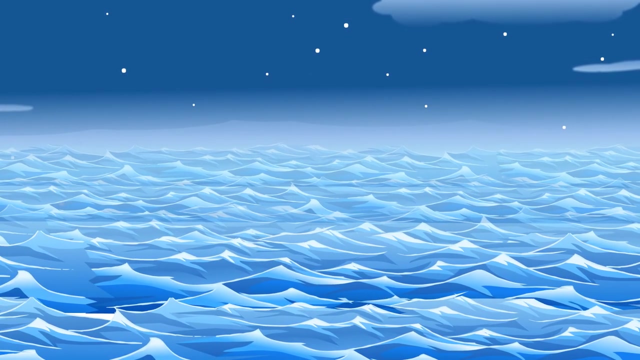 Inhale the waves rise And exhale. let the waves rise, Exhale the waves fall. Take some calming ocean breaths in and out at your own pace. You can even imagine your belly is filled with water, blue water, like the ocean. 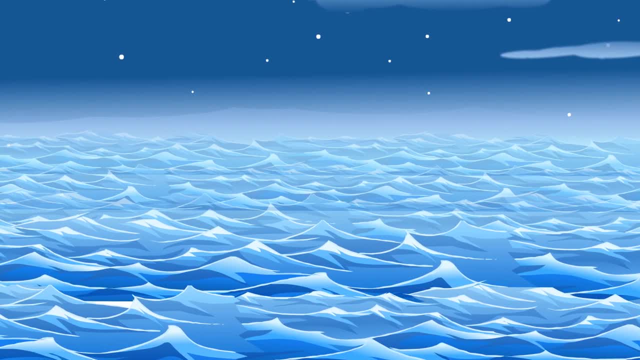 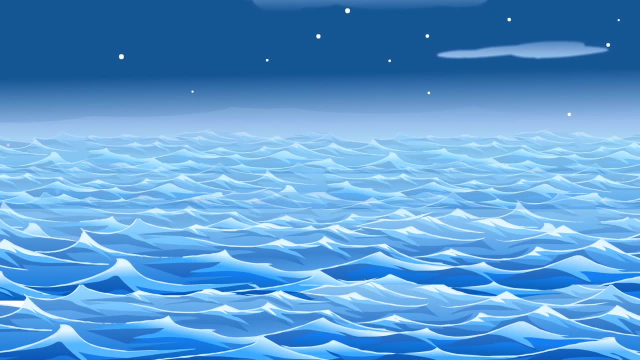 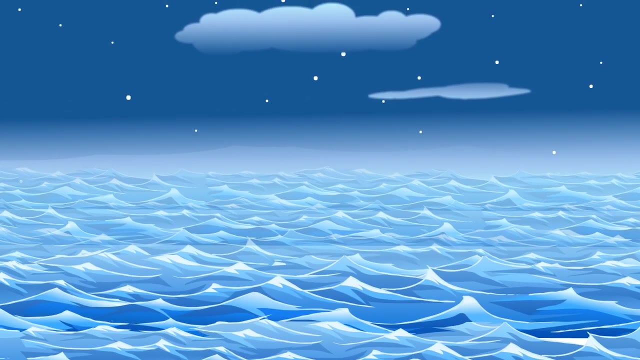 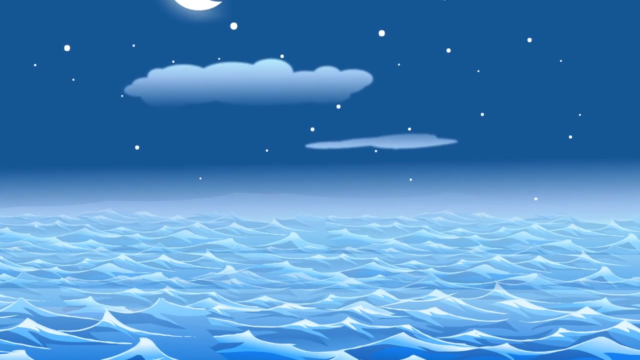 Take some relaxing baths here. Inhale- let the waves rise. Inhale the waves gently go up And exhale let the waves gently go down. Inhaling And exhaling, Inhaling. Maybe the moon begins to rise. 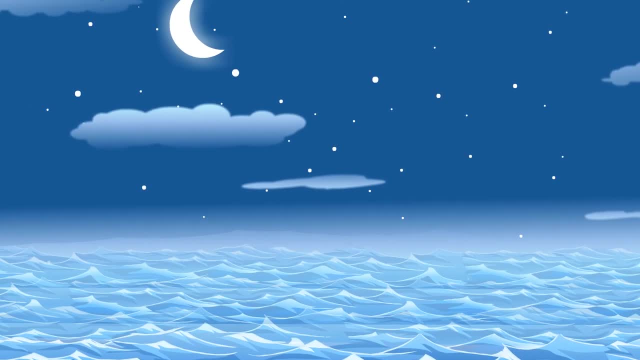 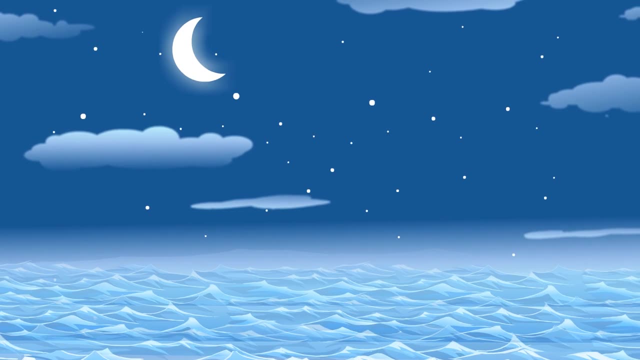 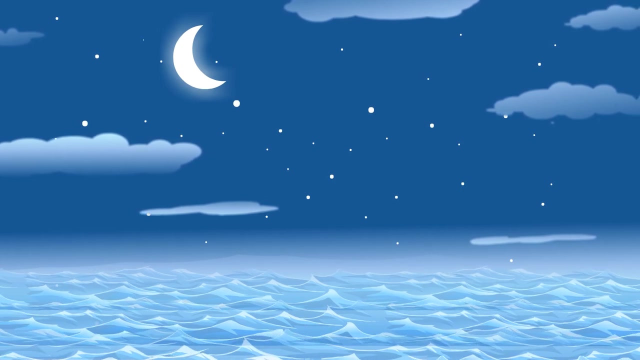 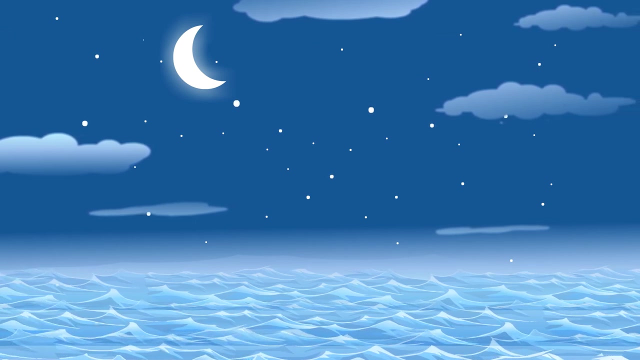 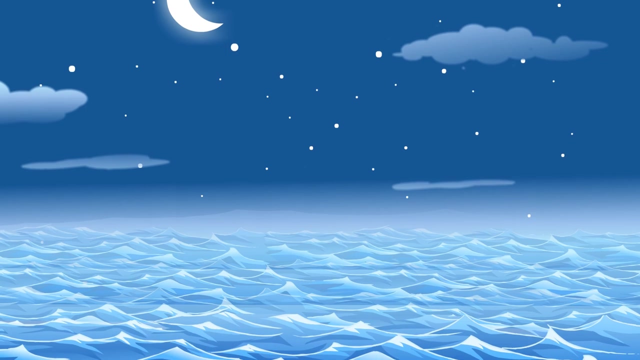 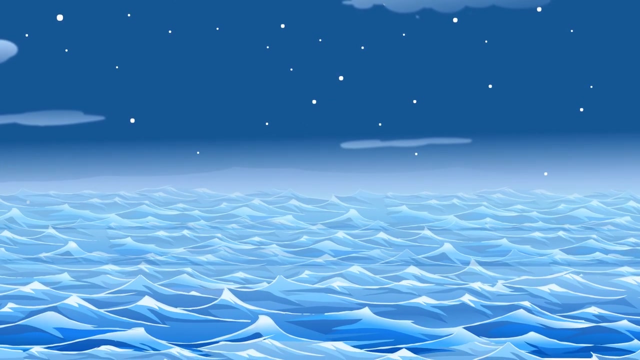 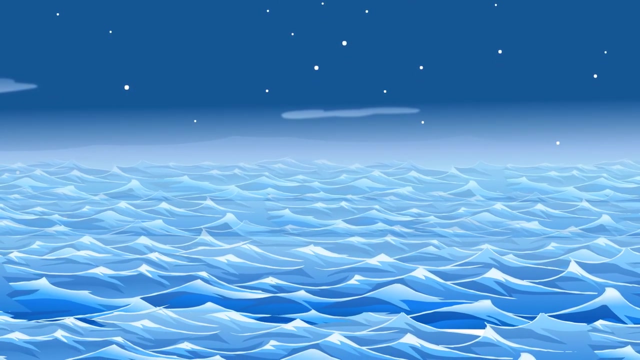 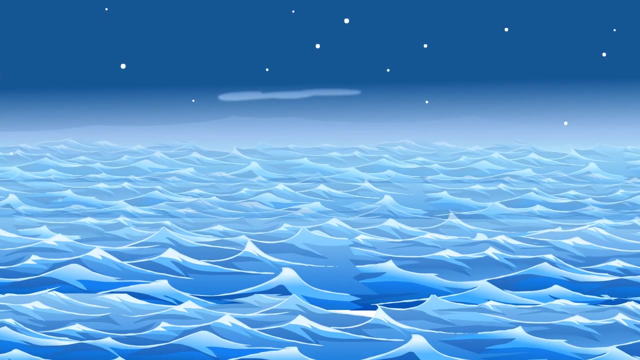 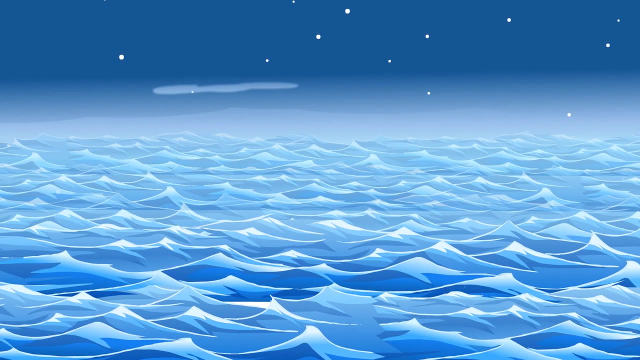 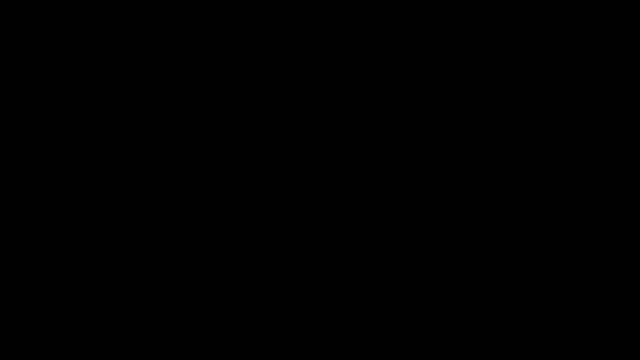 Maybe the moon begins to rise on your water belly like it pulls on the ocean and the tide. Take a few more ocean breaths and when you're ready you can open your eyes. Take a few more breaths and when you're ready you can open your eyes.